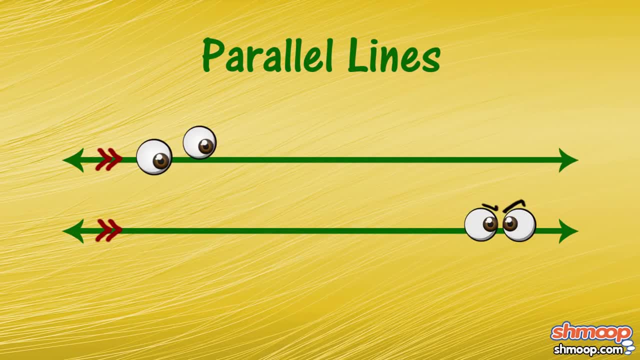 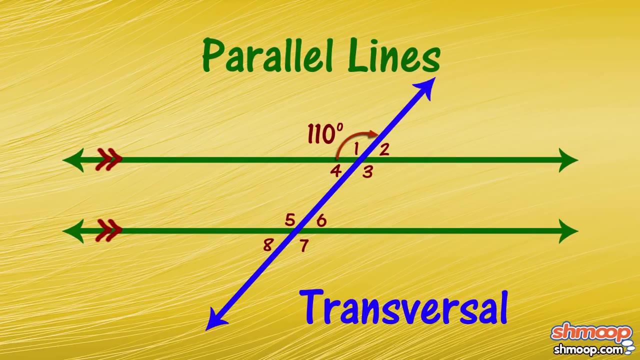 …parallel lines. Parallel lines never touch, but they always stand by their partner. Now, that's love. When a transversal cuts across two parallel lines, it forms eight angles. If the measure of angle one is 110 degrees, what are the measures of the other seven angles? 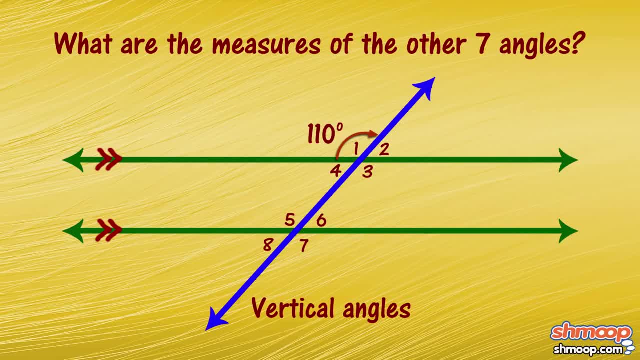 First, we can see that angles one and three are vertical angles, and we know that vertical angles are always congruent, In other words, they have equal measurements. So angle three has a measure of 110 degrees too. It also helps to know that corresponding angles…. 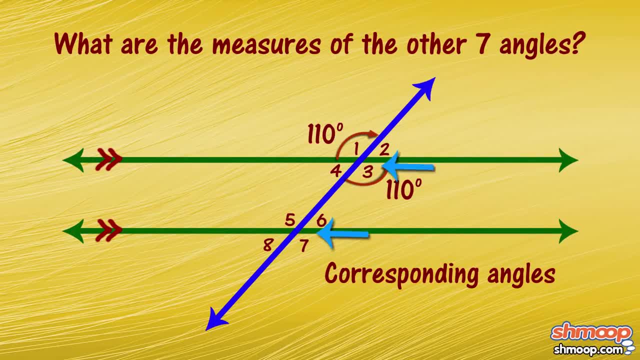 …or angles that are in the same position relative to the parallel lines and the transversal…. …are also congruent. In this case, the corresponding angle to angle one is angle five. So angle five is also 110 degrees. Wait…. 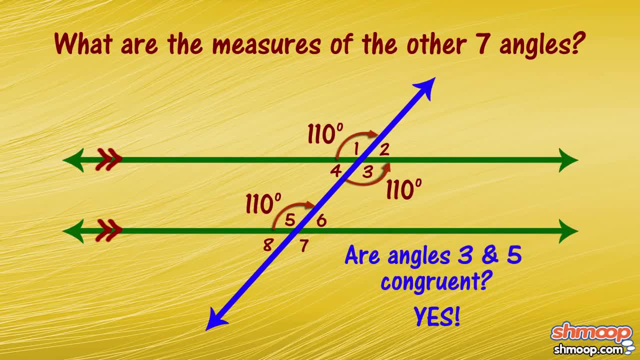 …so angles three and five are congruent too. Actually, yes, They're both on the interior, between the two parallel lines, and on alternate sides of the transversal. So we call them alternate interior angles. All… …alternate… …interior…. 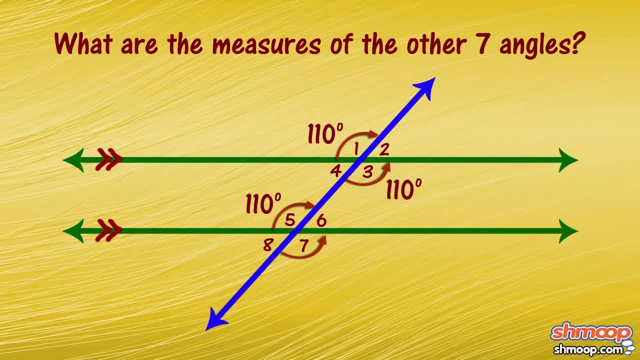 …angles… …are… …congruent. And there's one more angle that's 110 degrees and that's angle seven. Angle one and angle seven are both on the exterior of the parallel lines and alternate sides of the transversal, and they're called alternate exterior angles. 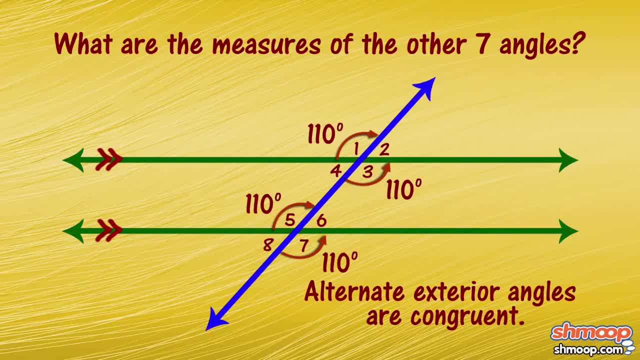 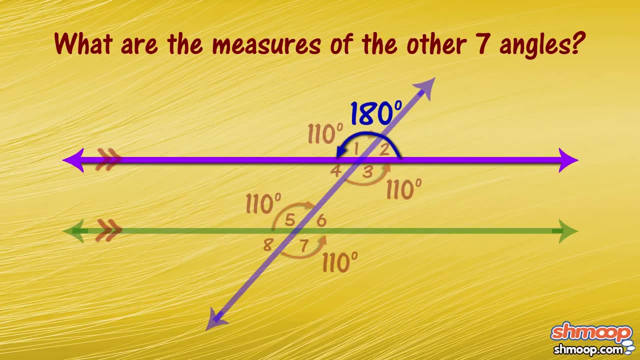 Alternate exterior angles are also congruent and we can check that using vertical angles or corresponding angles. Yep, looks like 110 degrees to us. Those are all the odd angles, But what about the evens? We know that a straight angle or a line has 180 degrees. 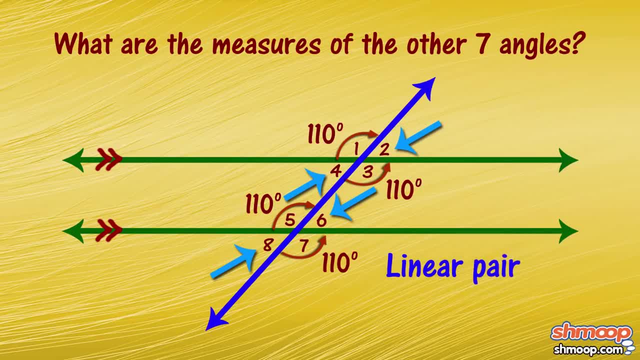 Since any even angle makes a linear pair with an odd angle. any even angle is supplementary to an odd angle. That means the even angles have a measure of 180 minus 110, or 70 degrees, And ta-da… …you now have all your angles.